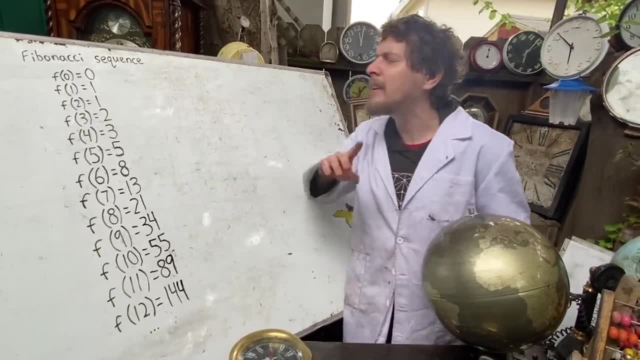 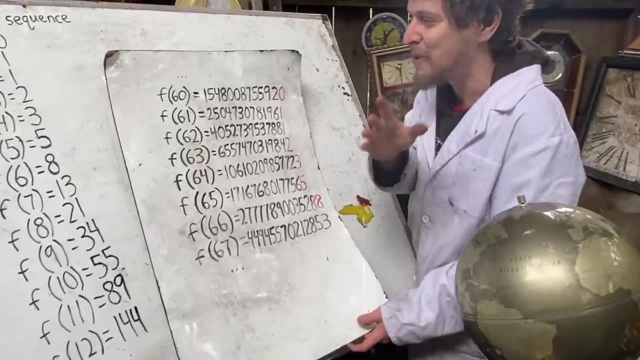 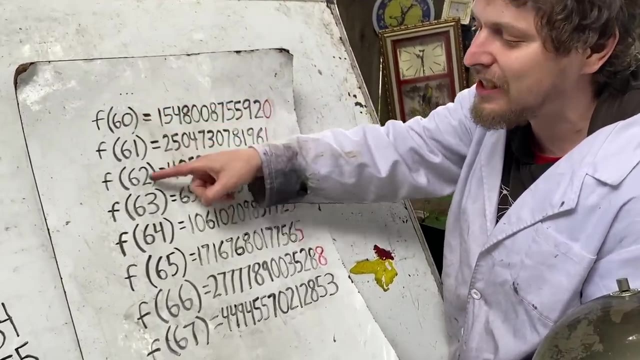 with all sorts of appearances. But if we jump ahead in the sequence a little bit, say to the 60th Fibonacci number, an interesting pattern emerges. I've highlighted the last digit of these Fibonacci numbers, from the 60th up through 66th, here red, because they look very. 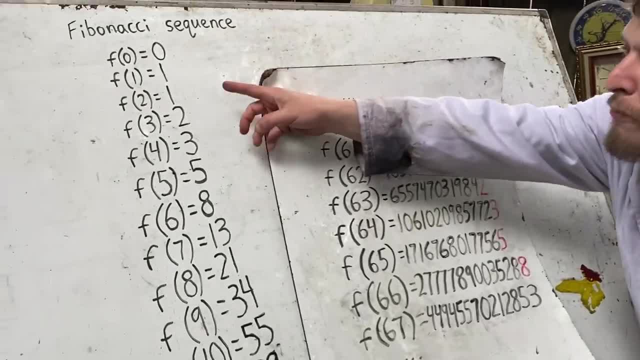 similar to the way the Fibonacci sequence itself began: 0, 1,, 1,, 2,, 3,, 5, 8,. 0, 1,, 1,, 2,, 3,, 5,, 8,. 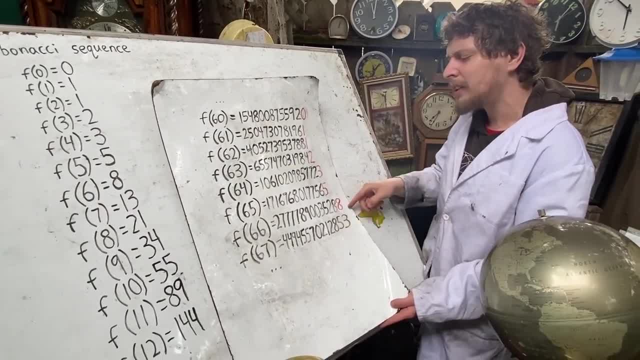 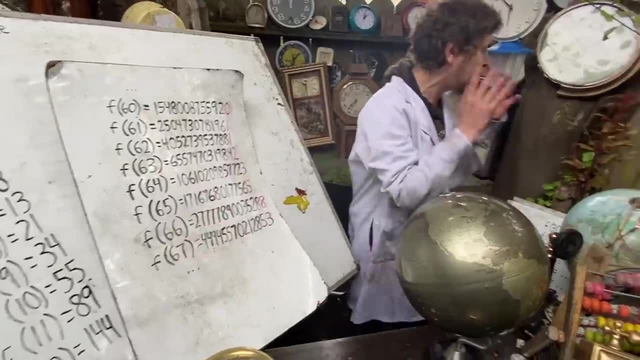 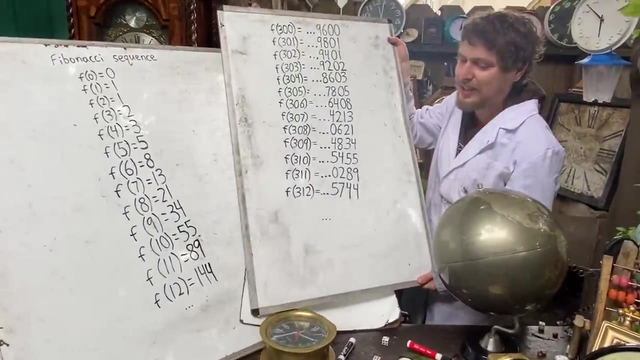 before it sort of overflows And the last digit didn't have enough room to contain that whole number. But if we jump ahead even further, say to the 300th Fibonacci number, where I've just written the last four digits of these Fibonacci numbers, from the 300th through, 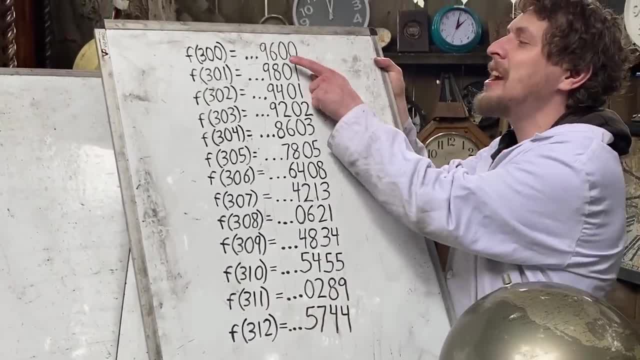 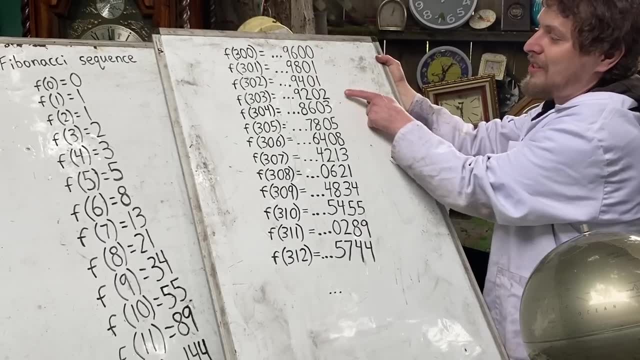 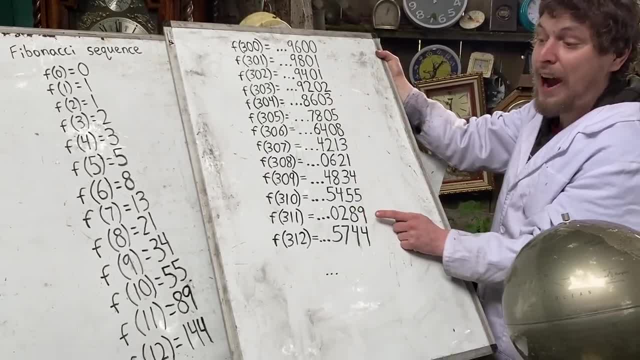 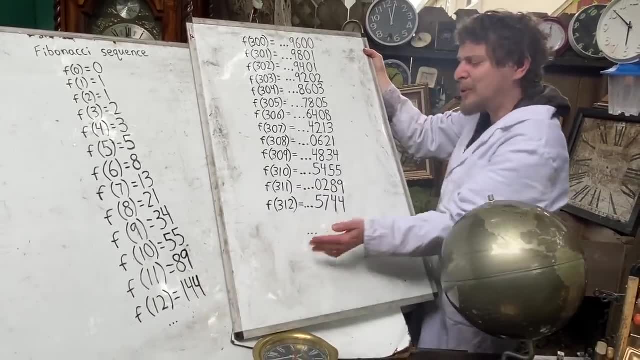 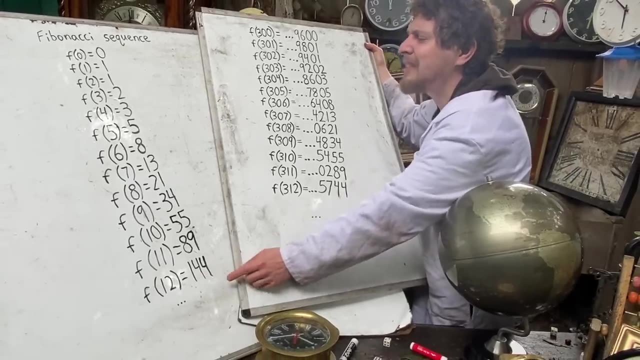 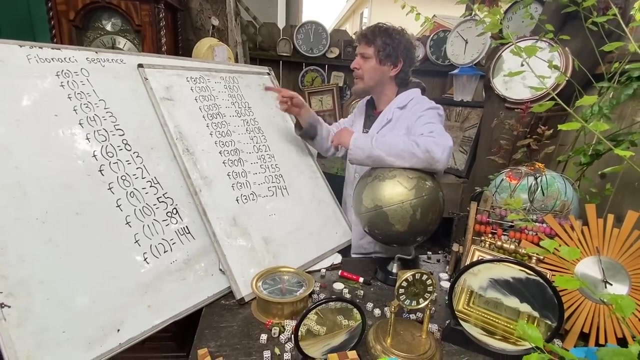 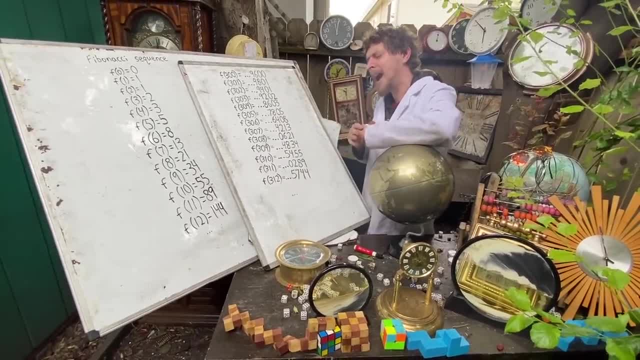 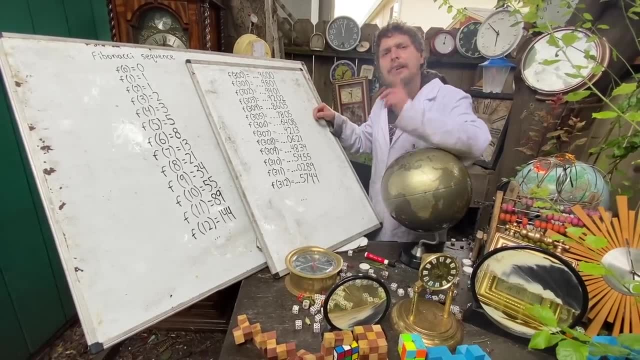 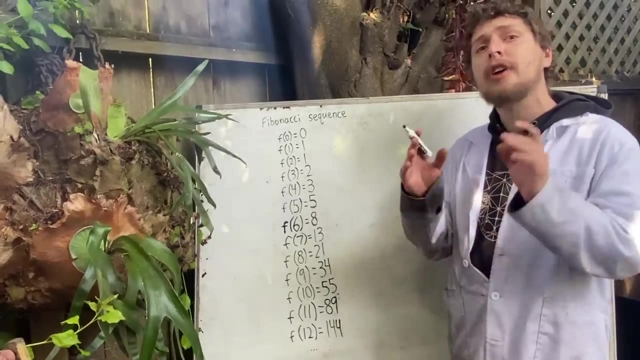 Is there room for more Fibonacci numbers to come back, And is this just a quirk of our base 10 way of writing numbers, Or what would happen in other bases? Let's start by seeing if the Fibonacci sequence has a pattern in terms of even and odd numbers. 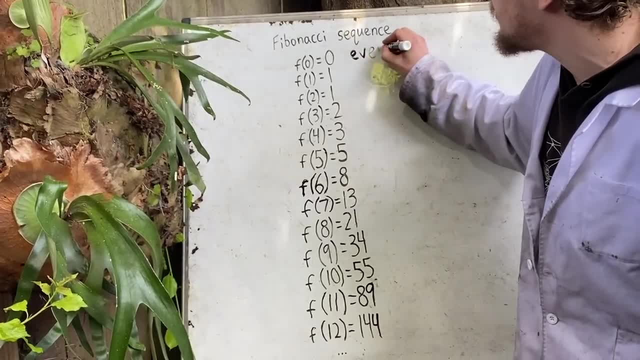 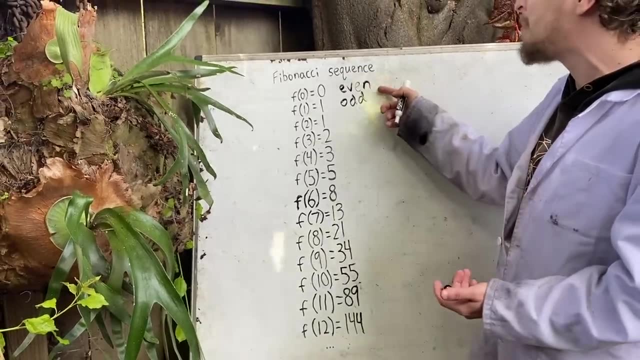 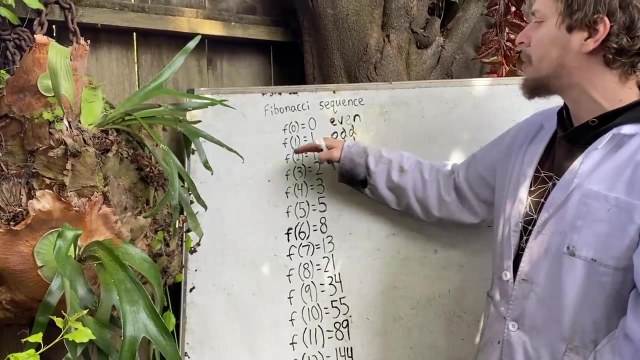 It begins with an even 0 and then an odd 1.. and even without knowing these further numbers, we can note that an even number plus an odd number always generates an odd number. And then the next term, which is determined by adding these two. 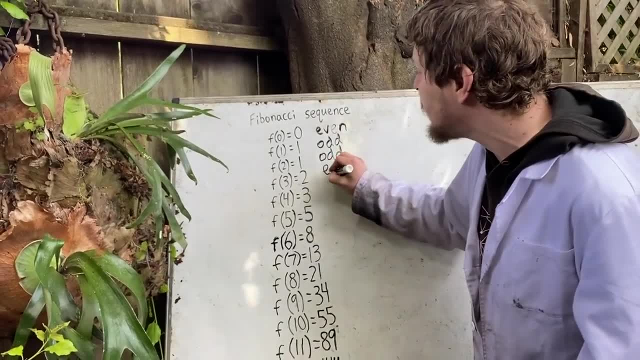 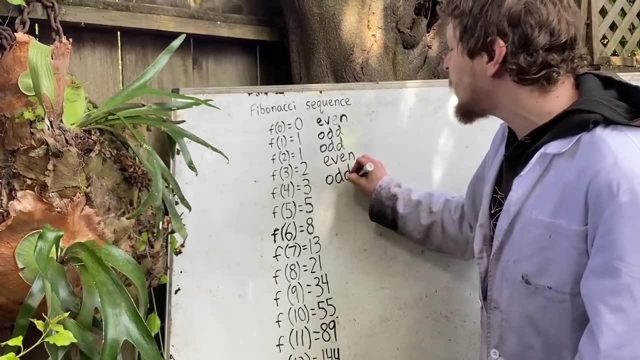 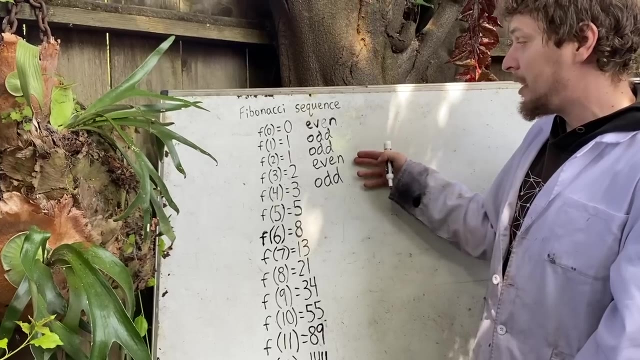 is an odd plus an odd, which is always an even, Then an odd plus an even is always an odd. And hey look, we're sort of back where we started, because this next one will be determined purely from even plus odd, just like that previous term had been determined by an even. 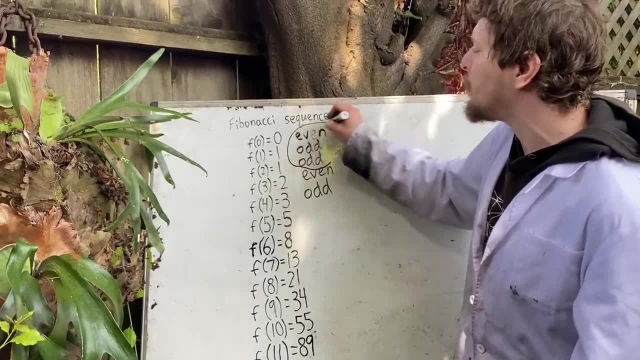 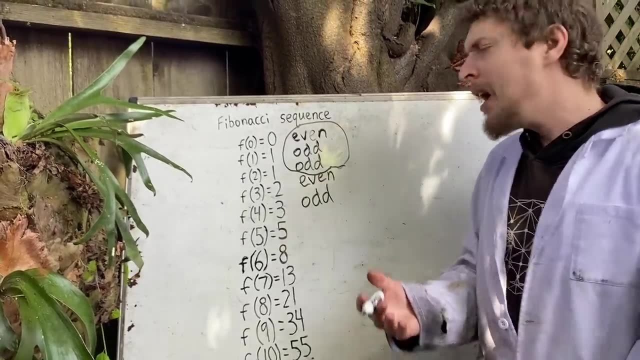 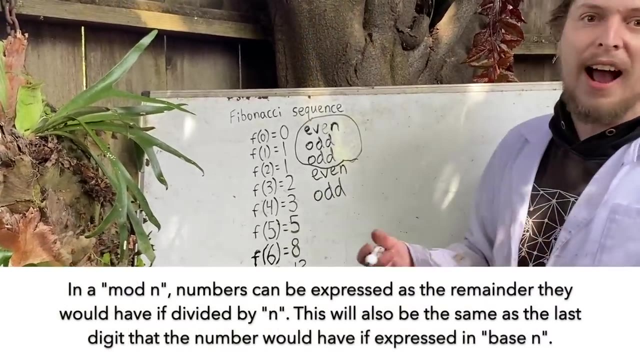 plus odd, And we can note that this part will loop as soon as we get back to a two in a row. that was at the beginning there And if we write this in mod two language, just writing the remainder, a number would have if we divided by two, where evens get a zero and odds. 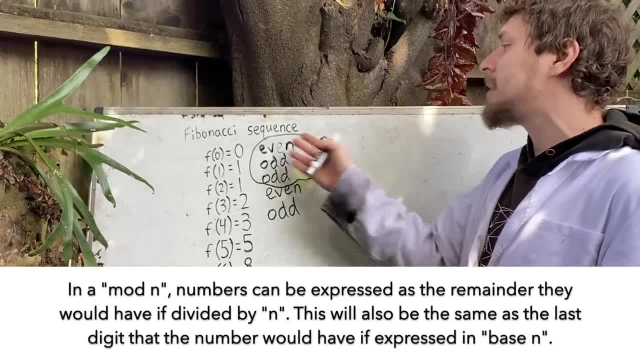 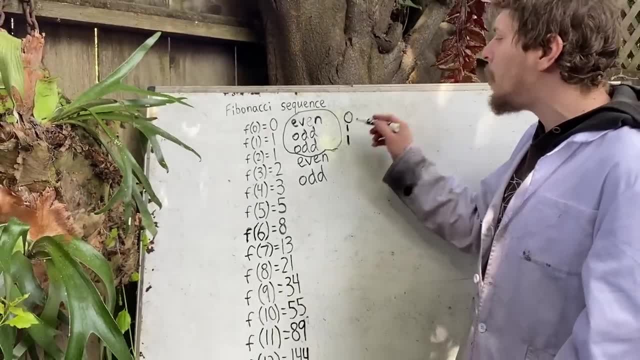 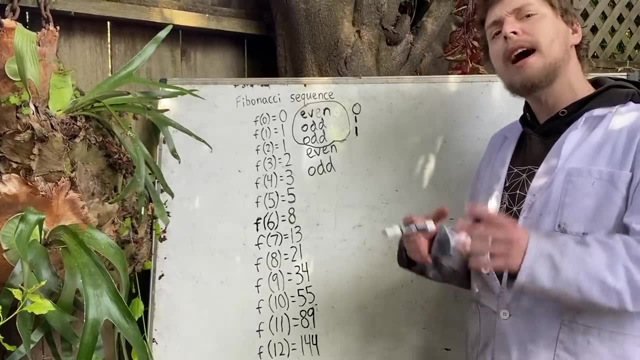 get a one which is also the last digit these numbers would have. if written in binary, the Fibonacci sequence will loop: zero, one, one, zero, one, one forever. So what about other mods or bases Like: how about mod 12? To see what patterns the last? 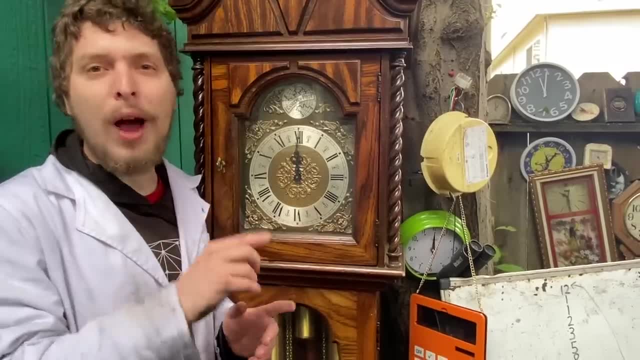 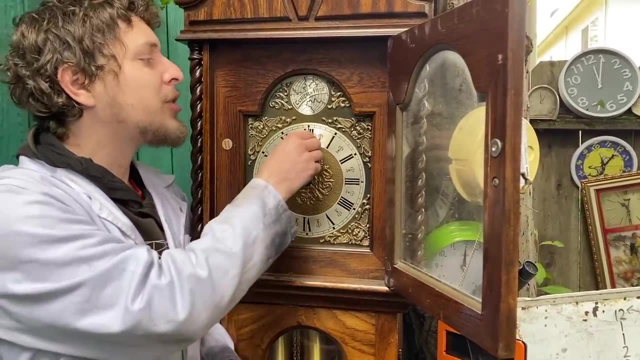 digit of the Fibonacci sequence might have in base 12,. we can use clocks as an example, a 12-hour clock. So if we had a clock like this and we would turn the 12s to zeros and the 10s and 11s, 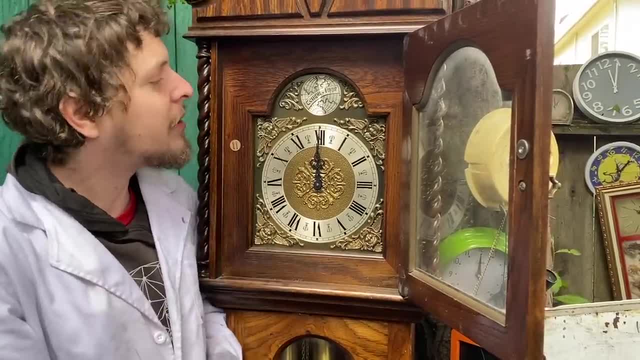 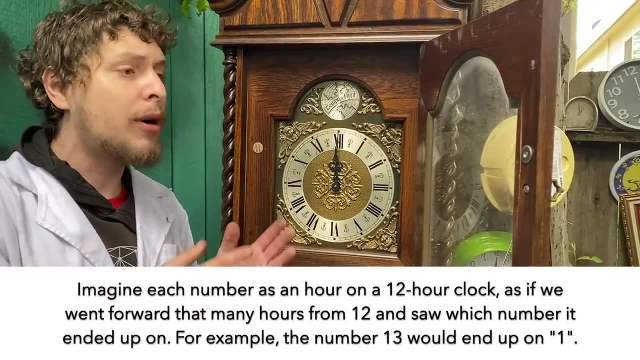 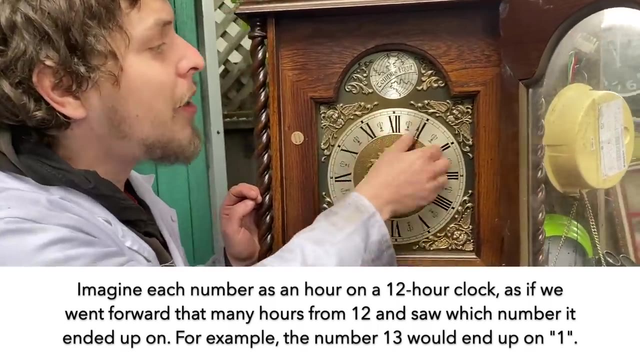 to single-digit symbols, if we were actually in base 12, and if we imagined going to an hour that was lined up with a particular Fibonacci number, like if my Fibonacci number was 13,, I would end up on the number one if I went that many hours from the top. Well looking. 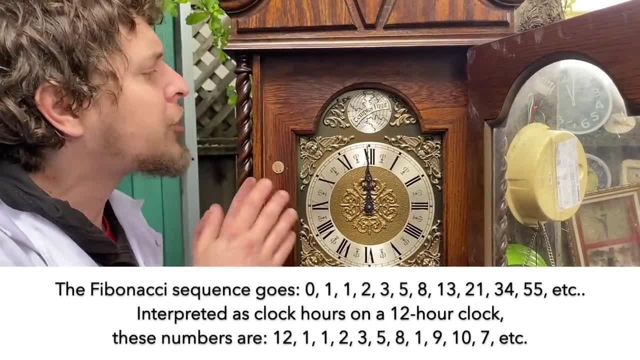 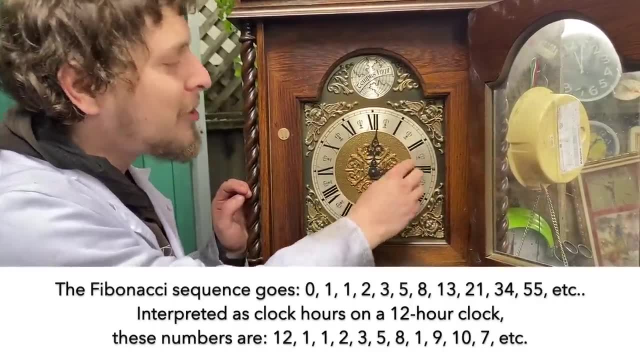 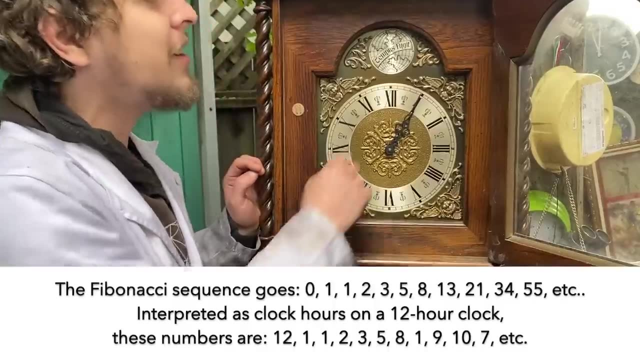 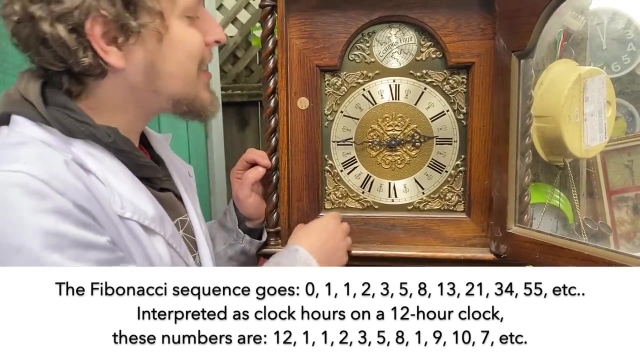 at which hours would correspond to which Fibonacci numbers? I would end up being at 12,, one, one, two, three, five, eight. the first few are pretty predictable, And then I would go to that 13,, then around to 21,, which would end up sending me to there, and so on, And 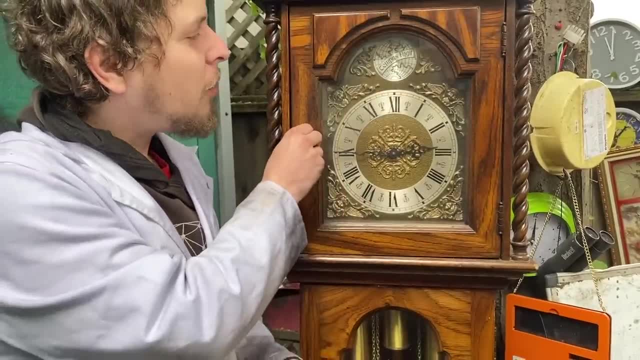 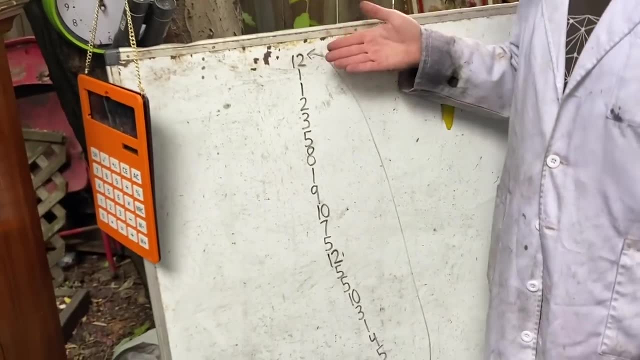 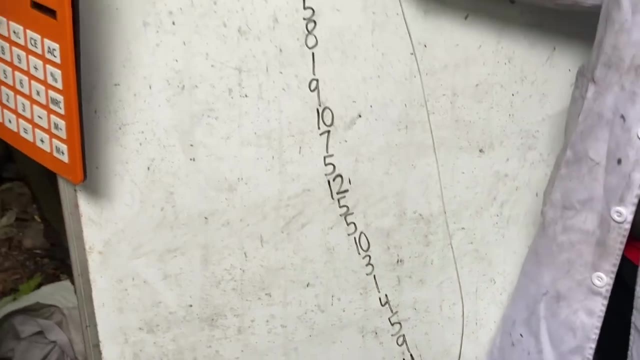 eventually I would hit a certain cycle Now where I was back to the pattern I had done before. here is the numbers that I would hit as hours playing that game, And after 24, I would return to a Fibonacci number being at 12, one being at one and 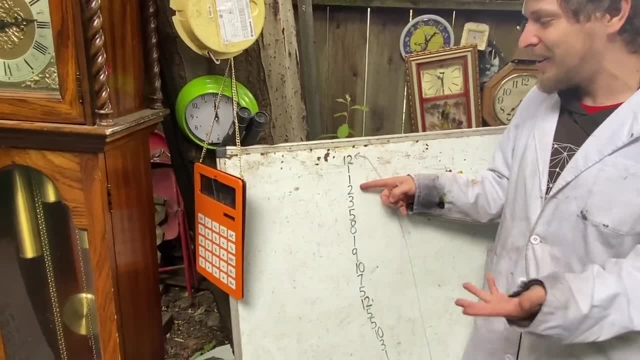 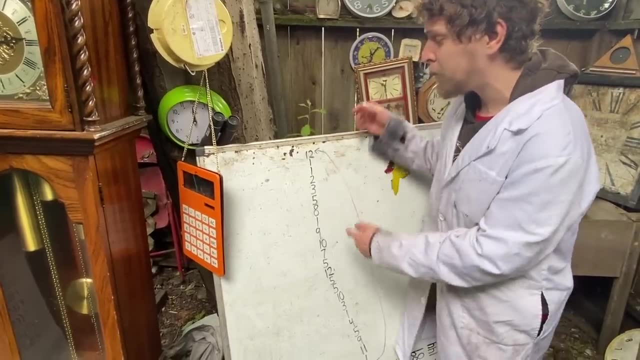 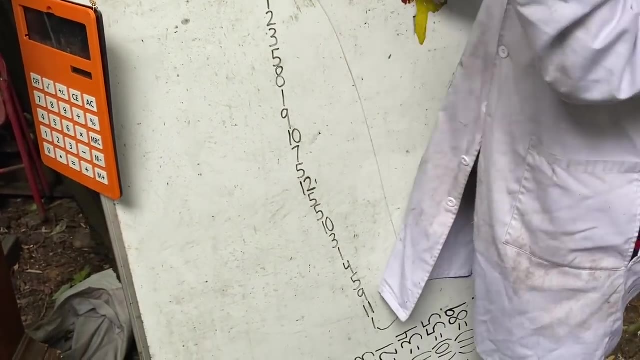 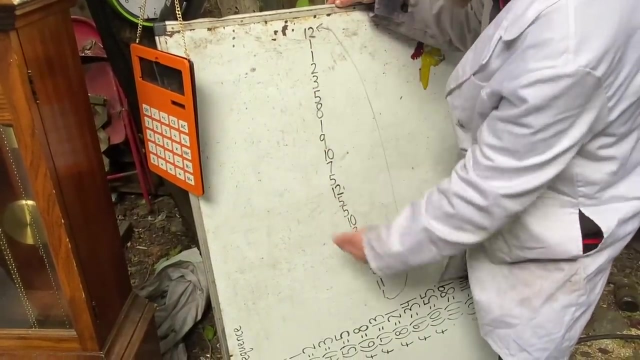 another one being at one, a Fibonacci number being on the hour two, and so on. This tells us that in base 12, every 24 Fibonacci numbers the last digit repeats in a cycle. We can also notice that the hour number six isn't anywhere in that cycle, meaning that no Fibonacci numbers ever. 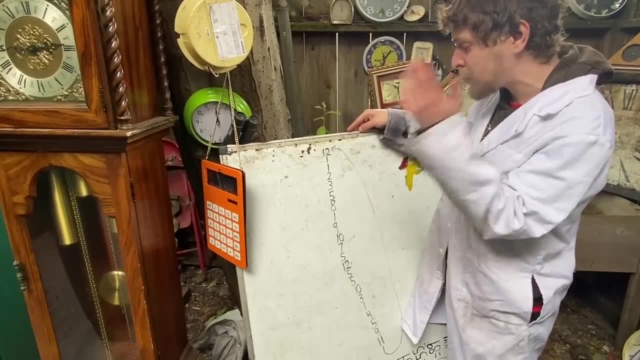 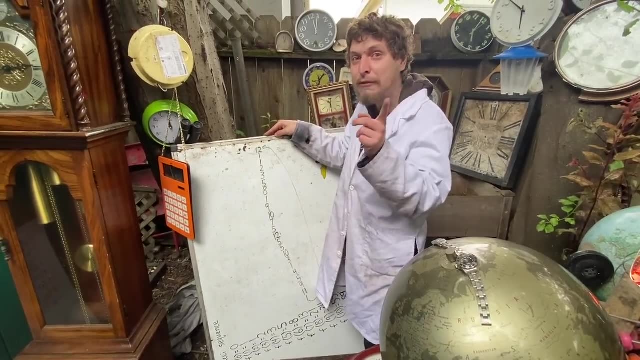 will end in the digit six if written in base 12, which also tells us that any Fibonacci number that's both threven and even must be at last 24 Fibonacci numbers. And that's exactly what we're looking for in the Fibonacci numbers. 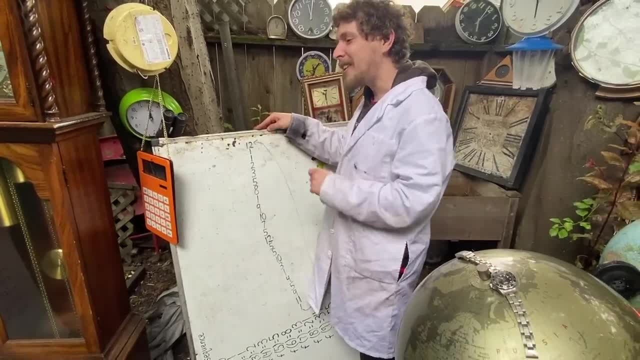 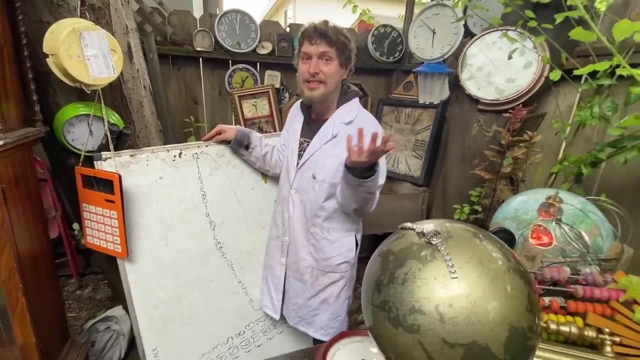 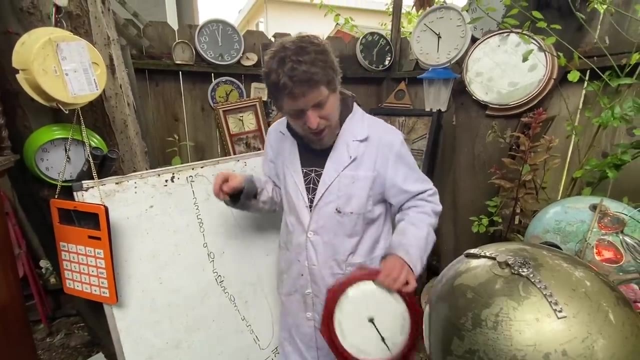 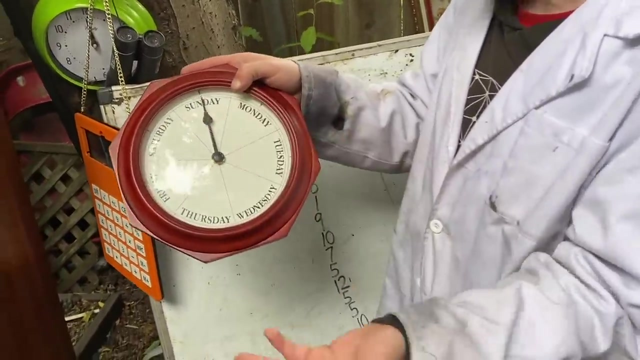 So if clocks can tell us things about base 12,- or we could have gone for 24 or 60, using minutes or other interpretations of hours- why don't we look at another common cycle of humanity, that is, weekdays, where every seventh day you're back on the same weekday? 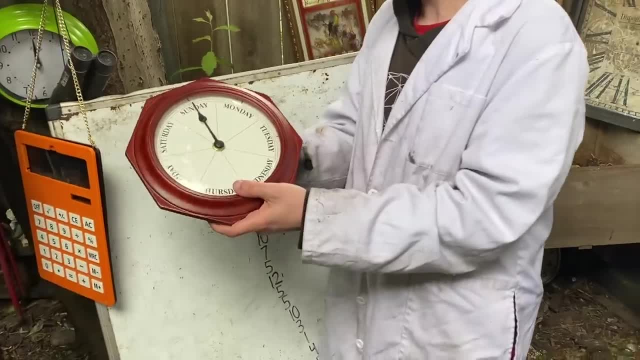 name like Sunday or Monday. Well, if I called a circle a weekday, it would be a weekday. Well, if I called a circle a weekday, it would be a weekday. I would send a certain one of these days zero, for example Sunday, and then I went. 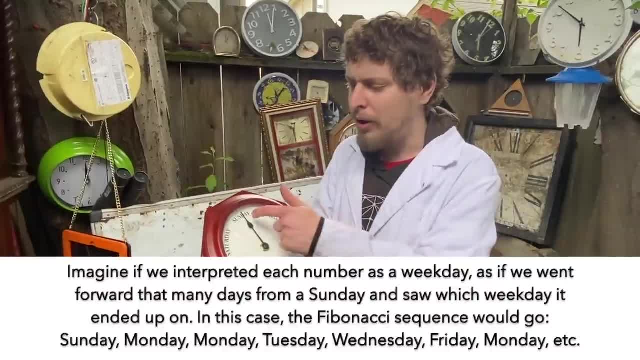 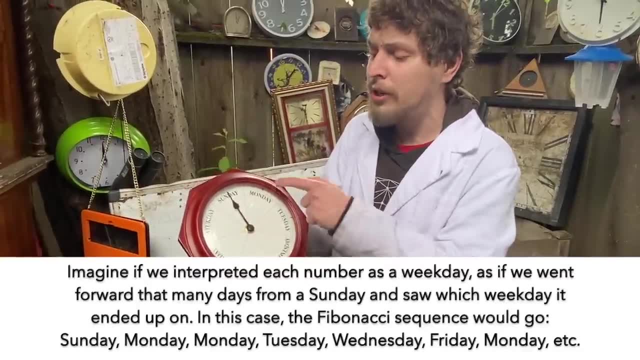 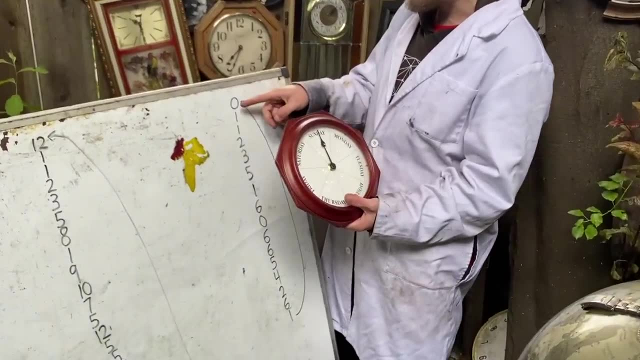 to the weekday that each Fibonacci number could be associated with. Like, if I had the Fibonacci number eight, eight days after zero would send it to a Monday. I would have a cycle there as well. I would land on the zeroth day. I picked like: Sunday here and Monday, Monday, Tuesday. 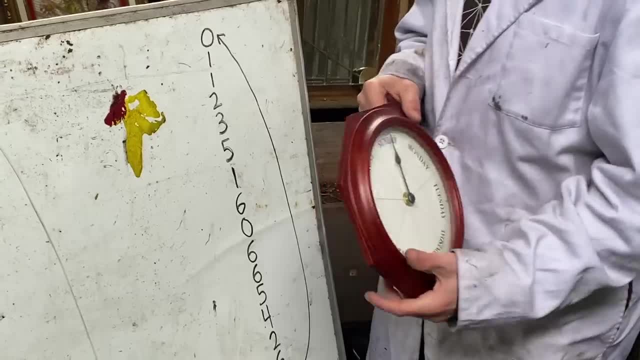 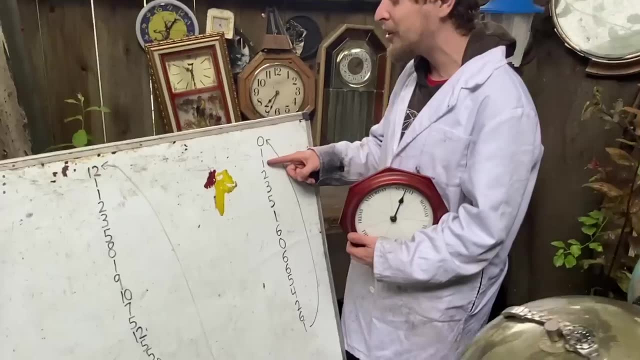 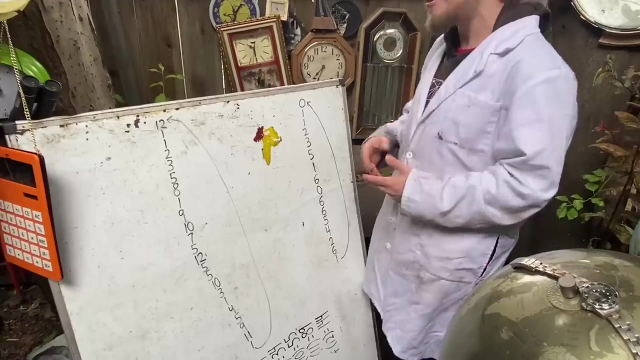 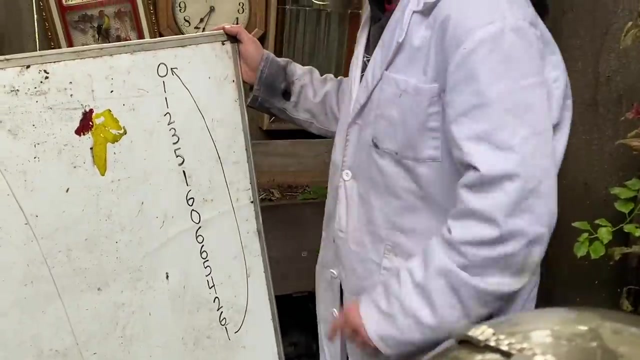 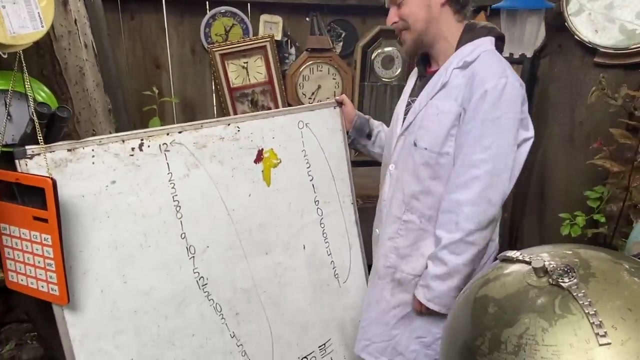 Wednesday, Friday, Monday, Monday, monday and etc. and every 16 fibonacci numbers. i would be back to the same pattern of weekdays that i started on, which tells us that in base seven, every 16 fibonacci numbers repeat their last digit in a cycle. so we can already see that 7 and 12, as far as bases, are even neater with this. 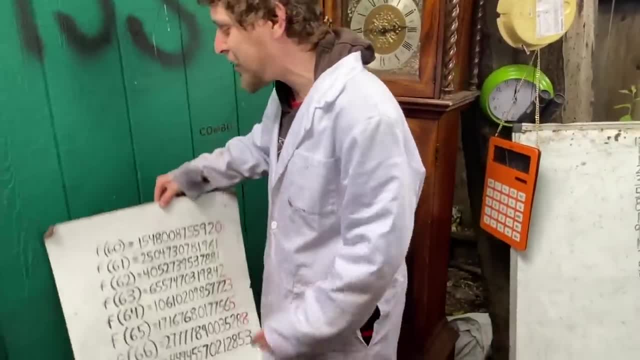 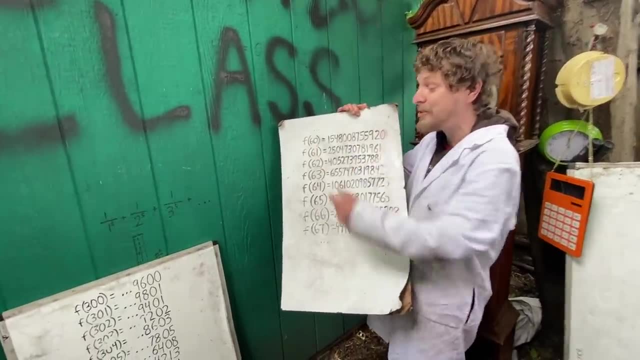 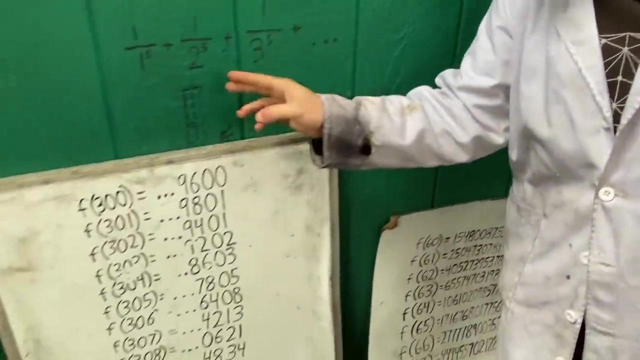 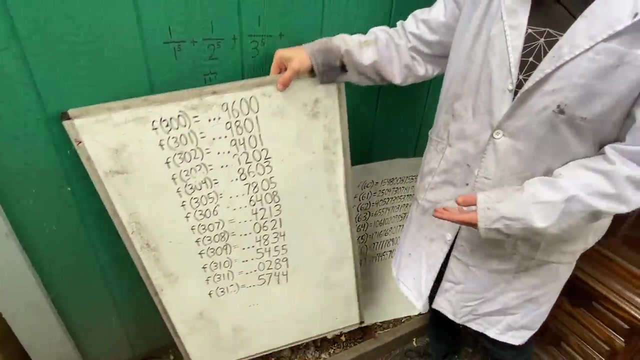 pattern of last digits than base 10, where the last digits loop every 60 fibonacci numbers, which is why i used that example. but we didn't just see the last digit here, we also made the last two digits do that, so let's jump into that. what does it take for the last two digits of a number? 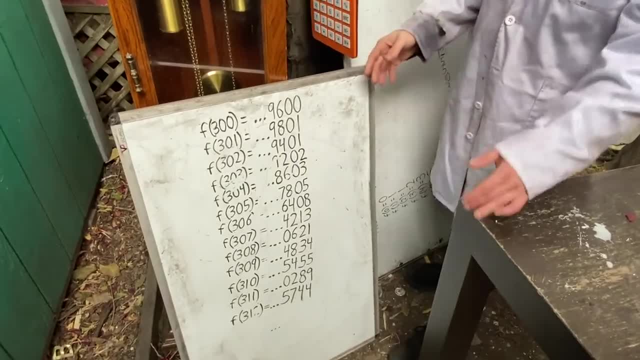 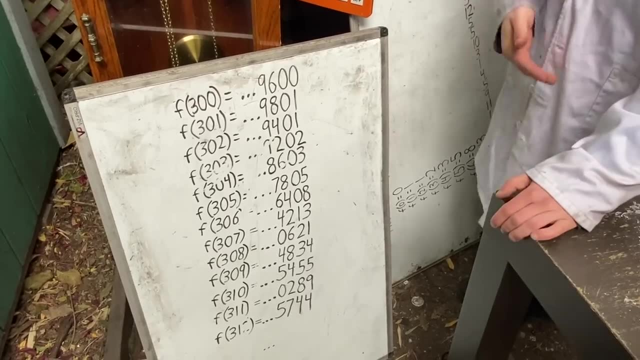 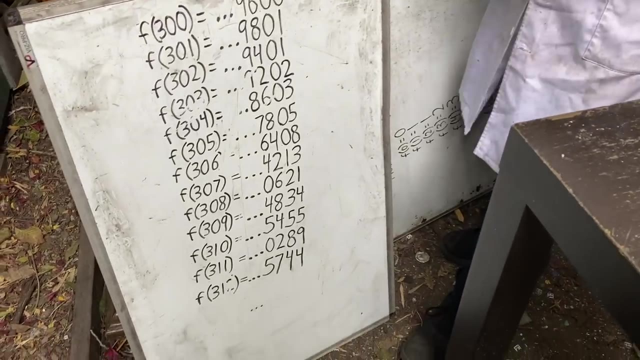 in base 10. to repeat: well, the last two digits cycle back around. if you were just counting up them: after 99, back to 0, 0 and every 100 numbers the last two digits. if you were just counting up them: after 99, back to 0, 0 and every 100 numbers, the last two digits. if you were just 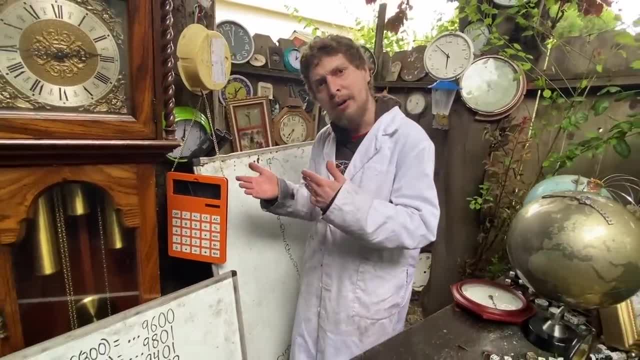 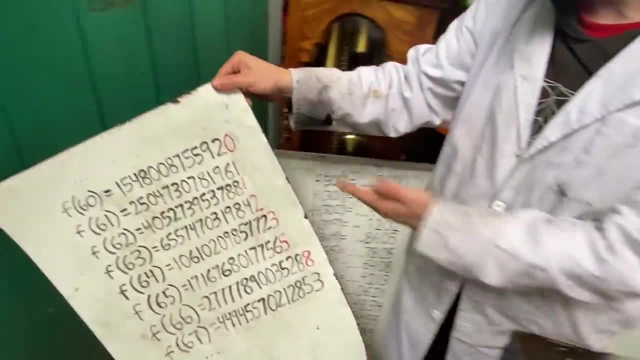 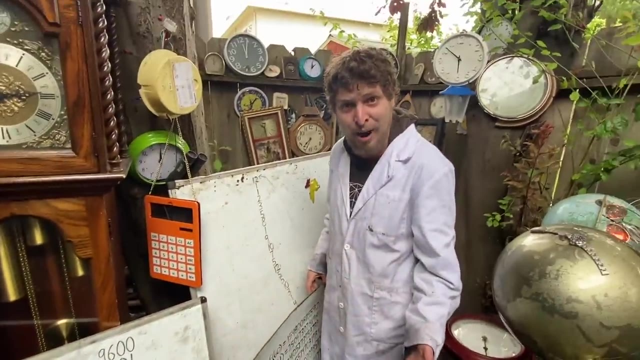 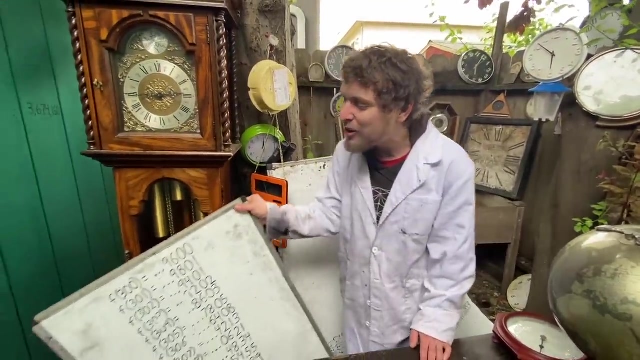 counting up a number line would loop back around. So just like the last digit of something in base 10 could be visualized like a 10 hour clock, the last two digits could be visualized like a 100 hour clock, like we're in what could be called mod 100.. And if we look at how the Fibonacci 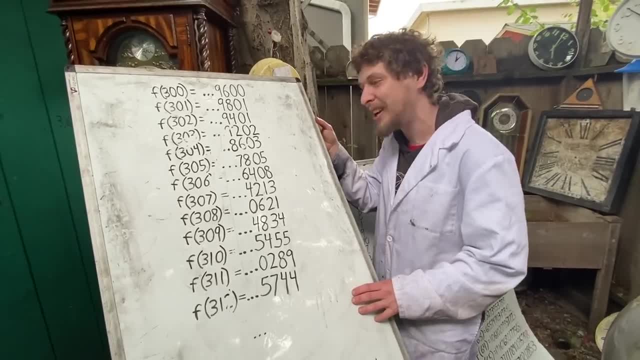 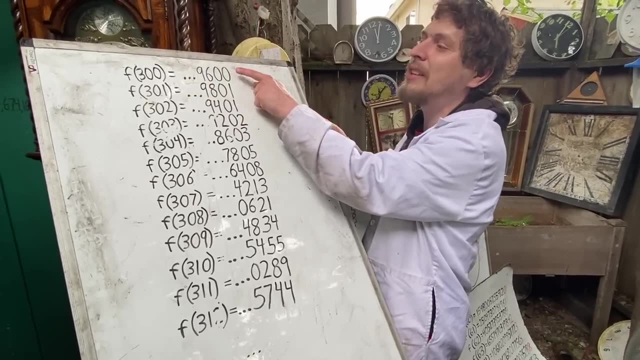 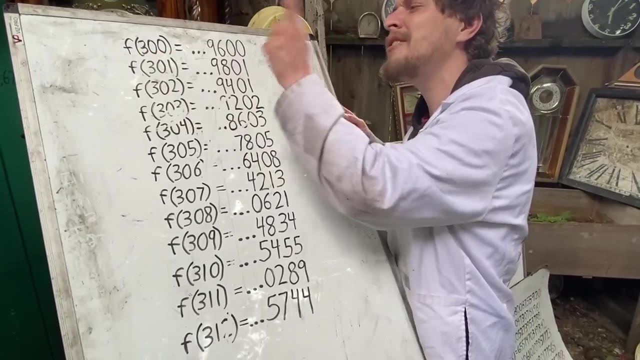 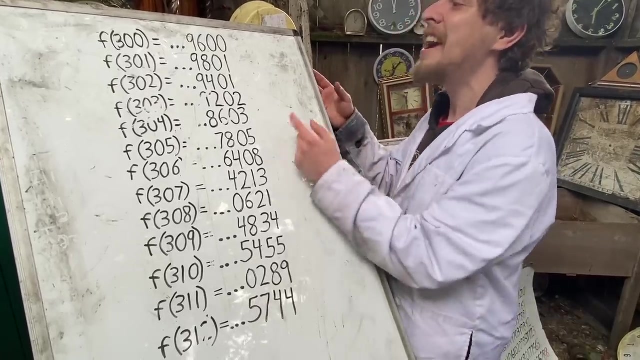 sequence acts in mod 100, or if we're in base 100, then these would all be smushed to smaller numbers and it would just be the last digit with 100 options cycling. Then it seems that at 300 we began hitting the same things. And it's true that in mod 100, every 300 Fibonacci numbers 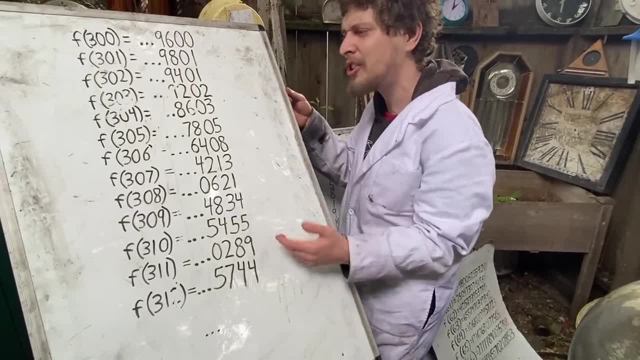 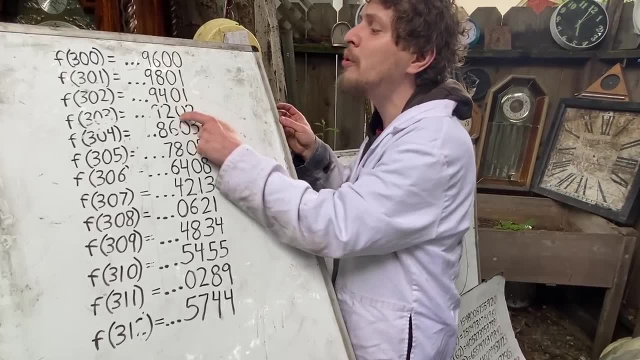 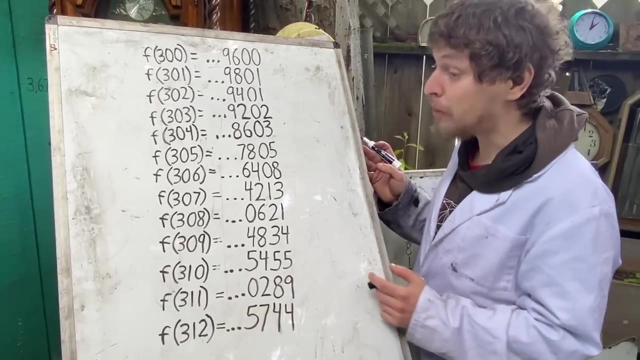 we will repeat The same result, meaning that every 300 Fibonacci numbers in base 10, we get two digits repeating in a cycle. Now, before we go further in the base 10 representations of Fibonacci numbers to see if there's a point where the last three digits repeat, let's ask a question which: 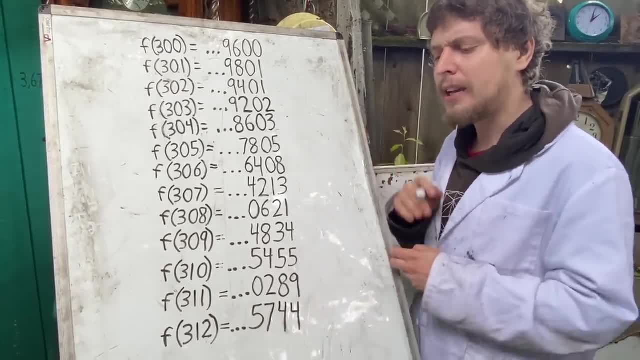 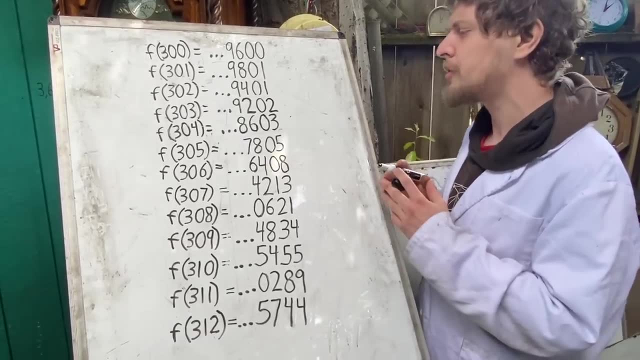 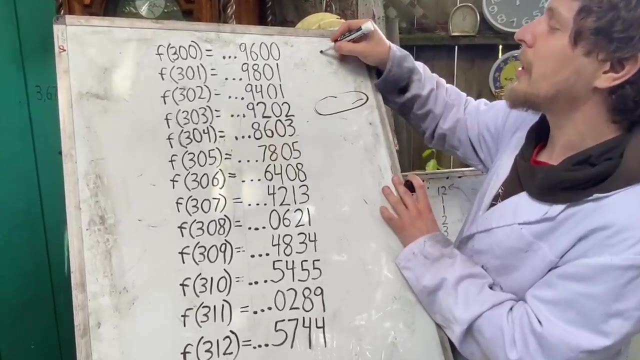 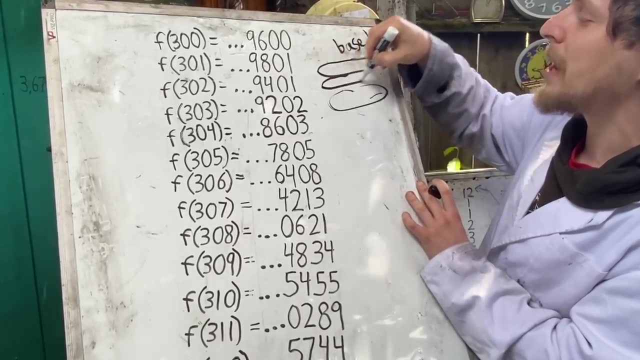 is for a given base and a given amount of last digits, will there always be a cycle or loop? Well, let's look at the last digit of a Fibonacci number in base B and note that the Fibonacci number is purely determined by the sum of the last two and that the last digit will: 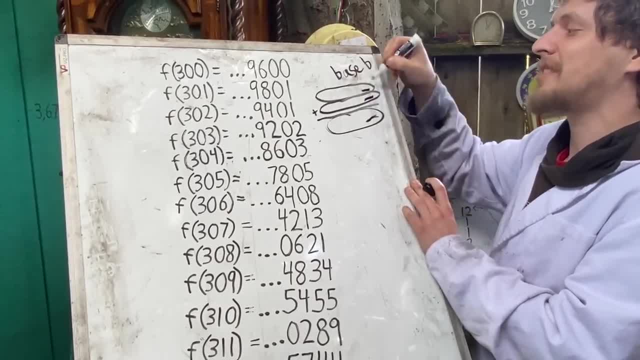 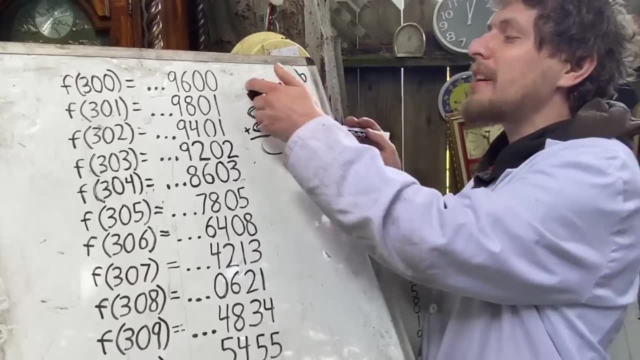 be purely determined by the last digits of the last two adding up, because all the further places in these numbers are the last digits that are adding up. So let's look at the. these numbers are too big of spots to affect that one's place, and so there's a finite amount of 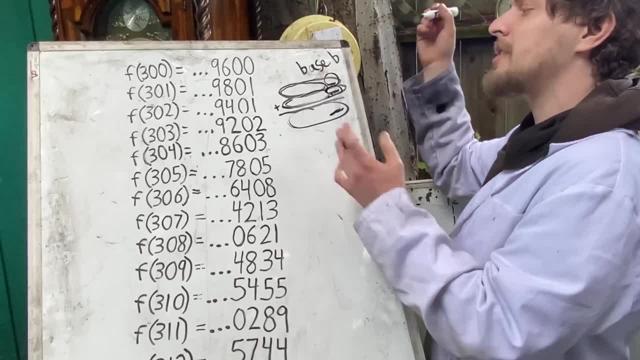 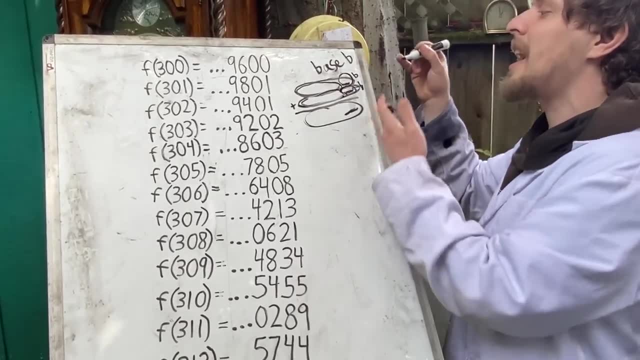 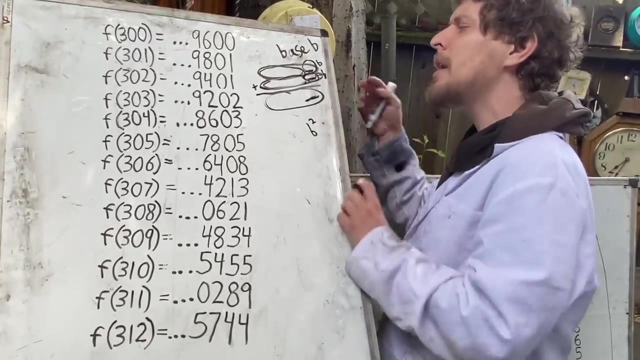 combinations of two final last digits, in fact that one has b options in base b, and so does that, leaving us with b times b or b squared, total possible combinations of two last digits in a row, and once those create the next last digit, that, with the second of those, will create a new. 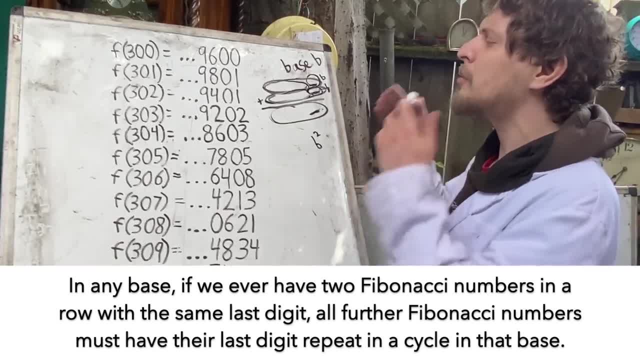 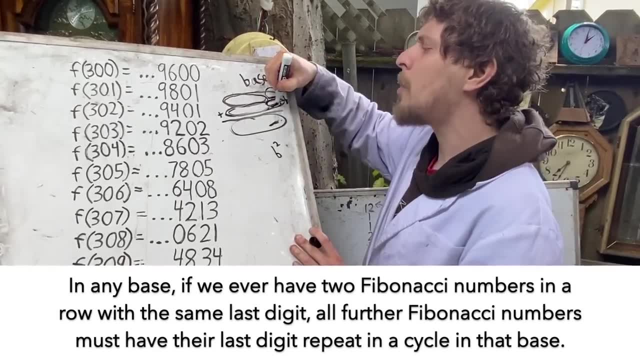 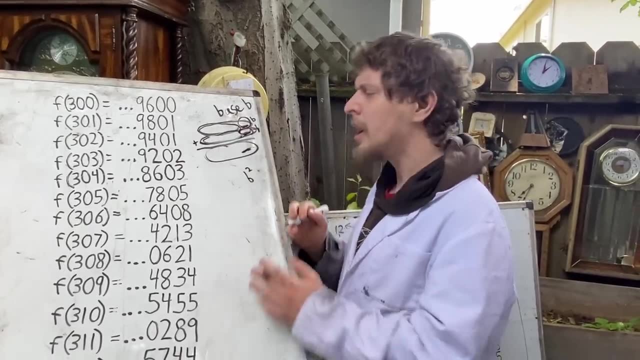 and keep going with the exact same pattern we've seen before, since each new one's place will be purely determined by the one's places of the last two numbers and there's a finite amount of combinations of those, even if we wondered about the last two digits in a base b. 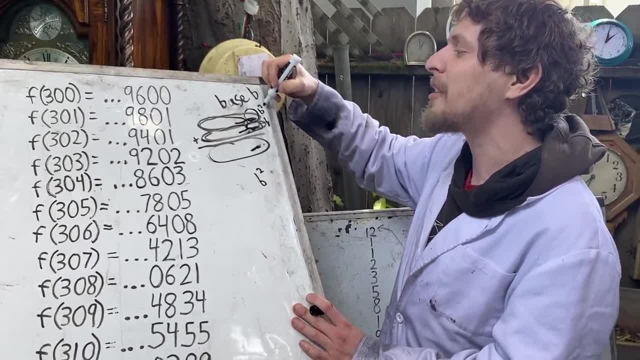 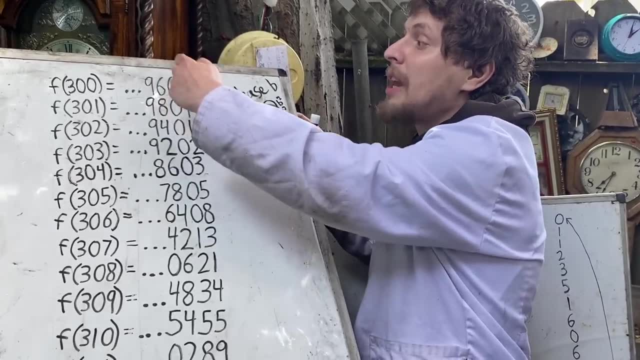 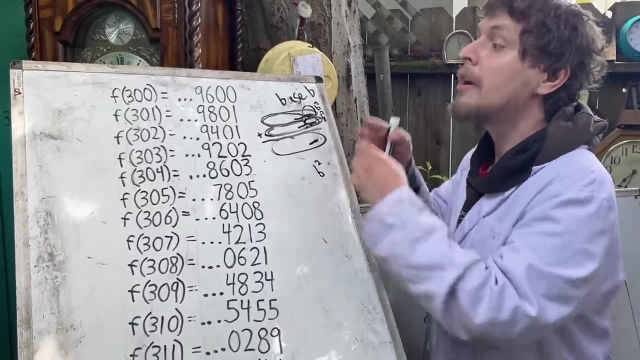 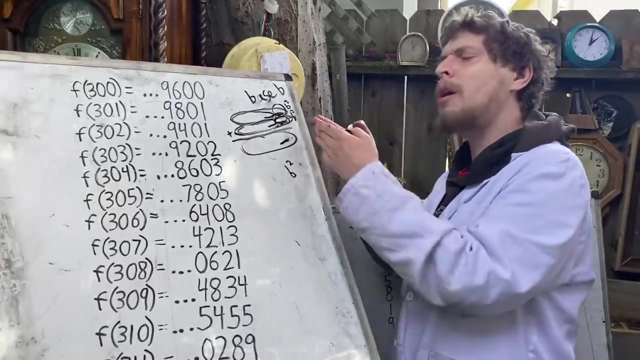 well you, there are b squared amount of options for each of those. for example, in base 10, to look at all the possible last two digit strings, from 0 to 99, there's 110 squared amount of possibilities, and so the total amount of possibilities of two strings in a row would be b squared times b. 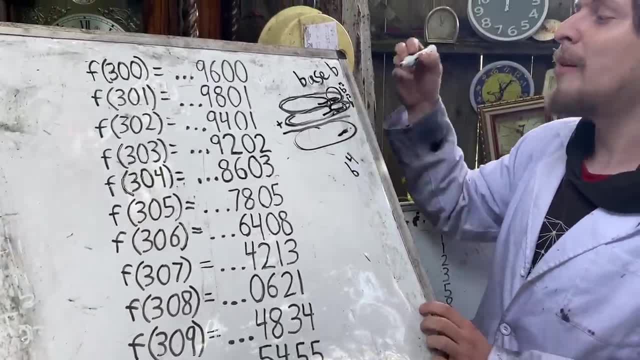 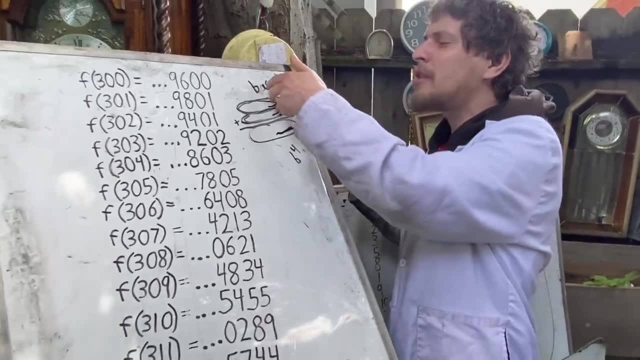 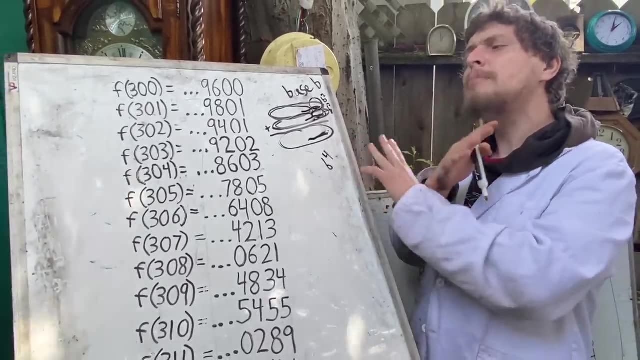 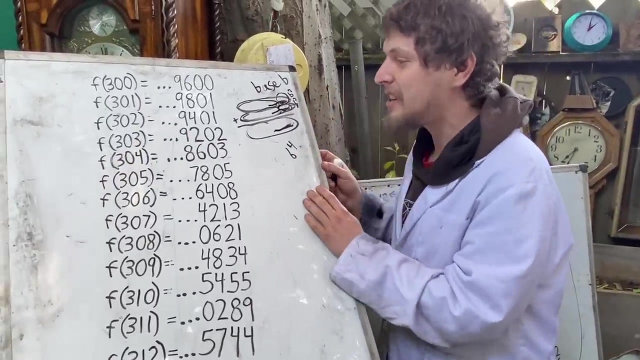 squared, or b to the fourth power amount of. so you'd think the number of electrons in some number gets reduced to b, even if we do a simulation where the infinity line of a number has to be the undefined, and that'd question the most redundant thing you can get out of the π讚jam condition. 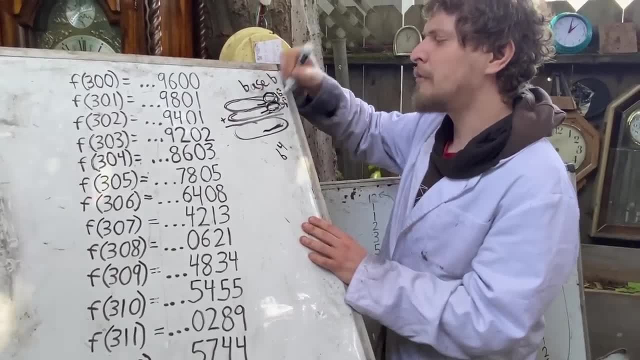 and so this is like a prohibition of the cycle that needs to be marked in order for us to solve. when we're done with ouraints and the deathoren blocks we zed. now we're going to need to keep in mind that we're going to need two�� rows of 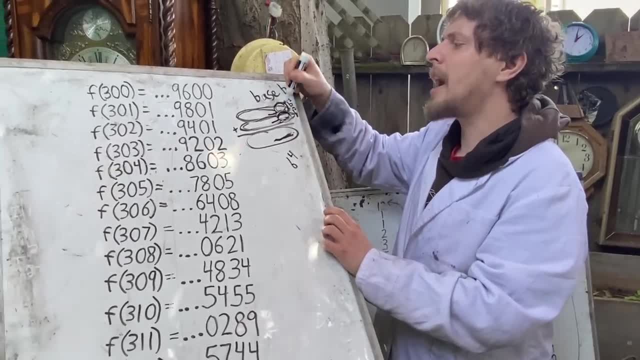 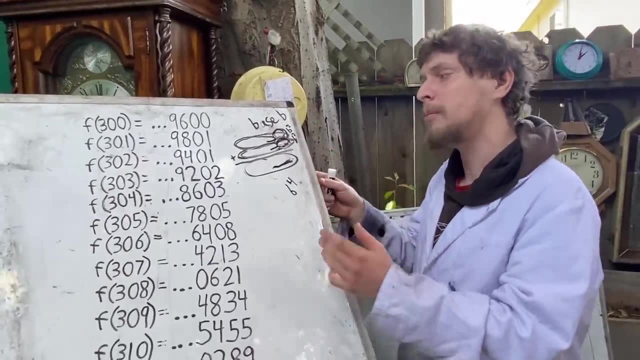 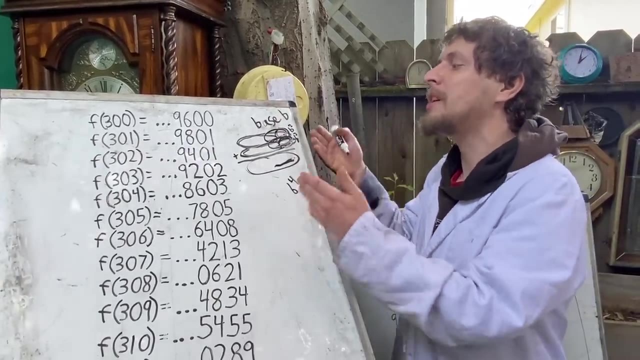 two SS's that have two digits in a base b, and this would be the only parts that could affect the new. last two digits of the next number must follow b times b- amount of possible options, and must cycle after at most b squared fibonacci numbers. the last two places are built off of b squared times b squared amount of options. 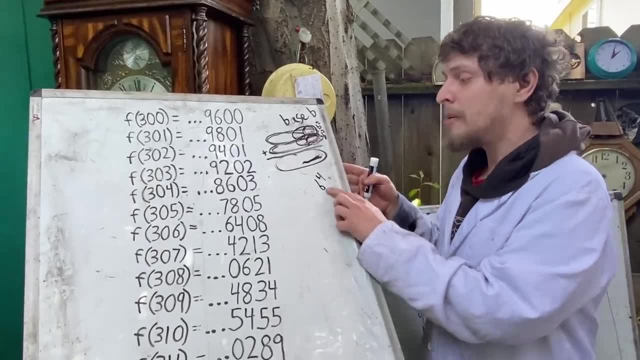 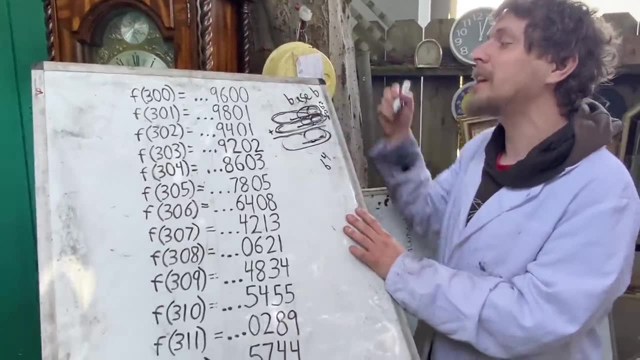 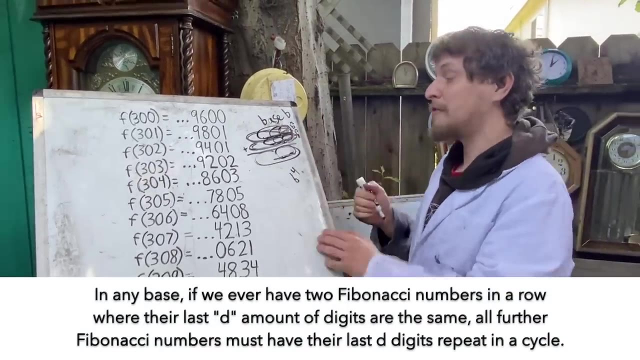 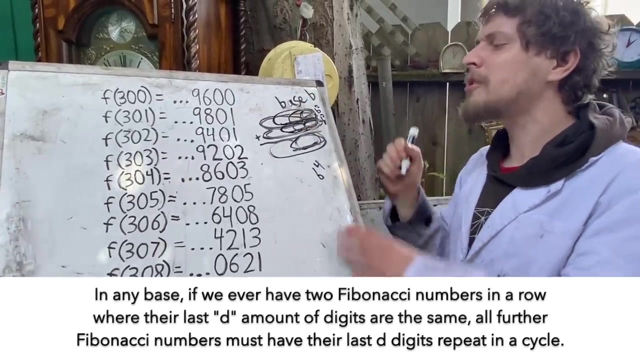 making them cycle at at most b to the fourth power amount of fibonacci numbers and for three digits, there would still be a finite amount of three digit ends there and three digit ends there, thus a finite amount of combinations of the last two three digit ends that leave us forced into 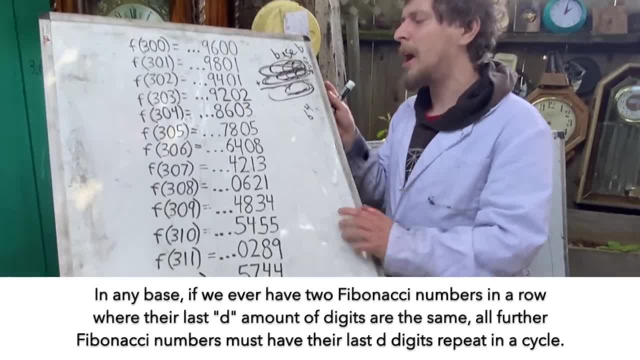 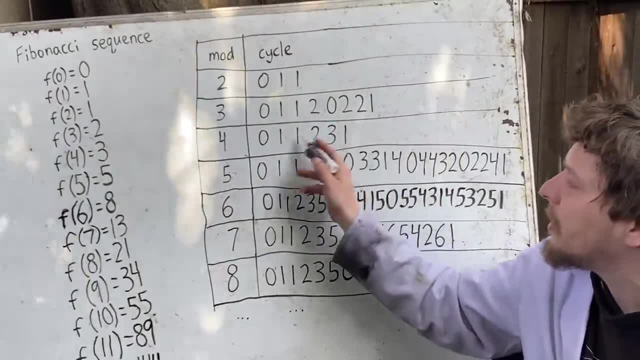 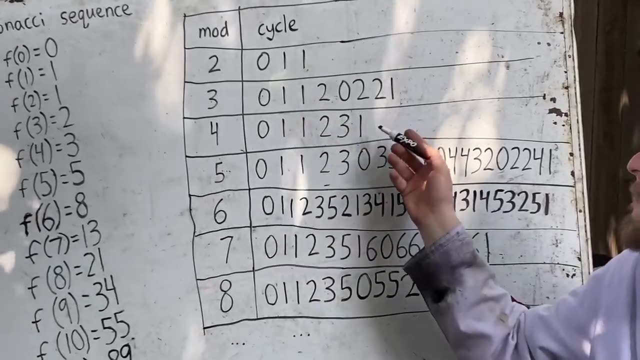 some sort of cycle for any amount of last digits in any base. here are the cycles that the fibonacci sequence loops in in different mods and these are also the cycles that the fibonacci sequence loops in in different mods- cycles of last digits that would repeat if we looked at the Fibonacci sequence in that given 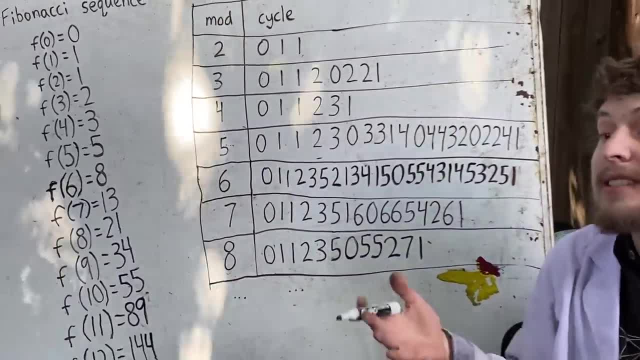 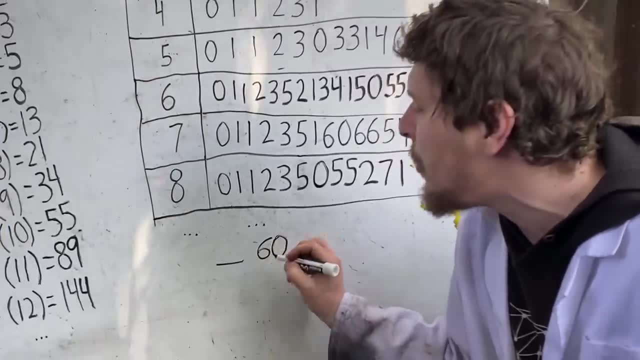 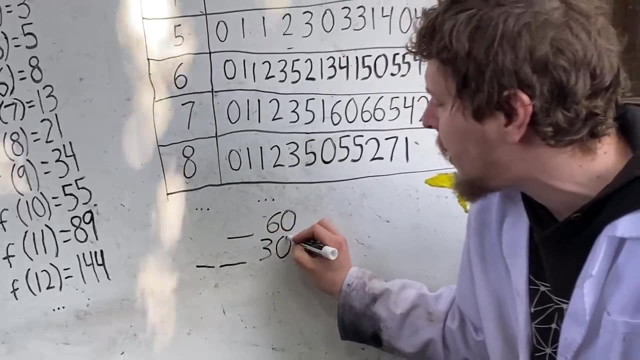 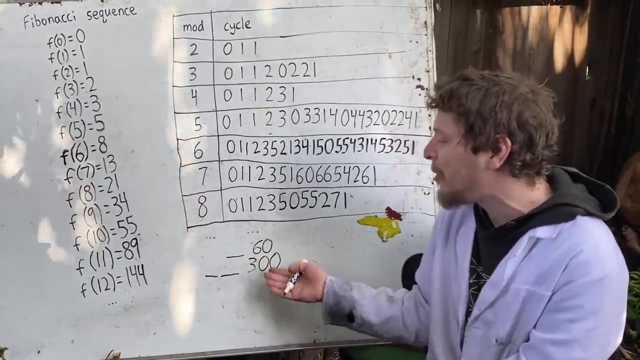 base and up in mod 10 or the last digit of base 10, we saw that the cycle was 60 in length and that we could also find a cycle of the last two digits that was 300 in length. that's because the mod 100 cycle is 300 numbers before it repeats and that could tell us about the last digit in. 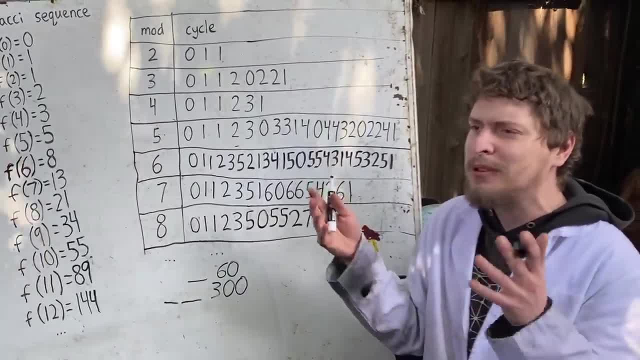 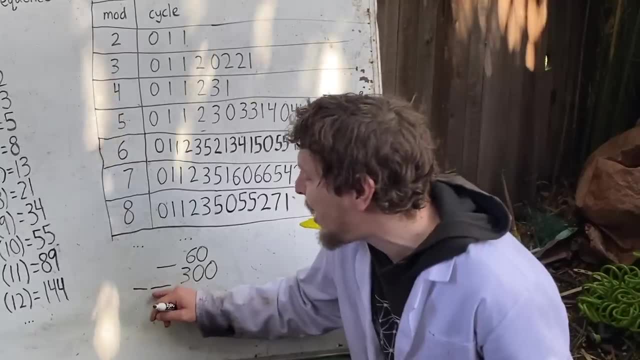 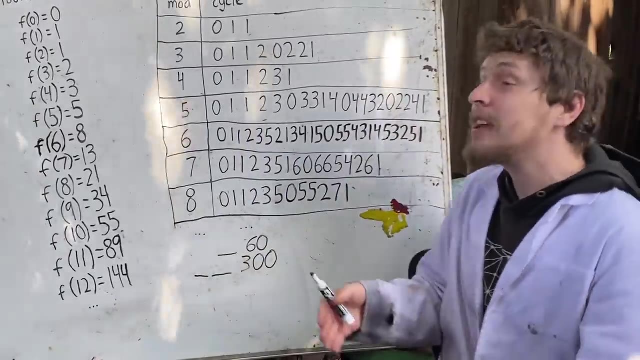 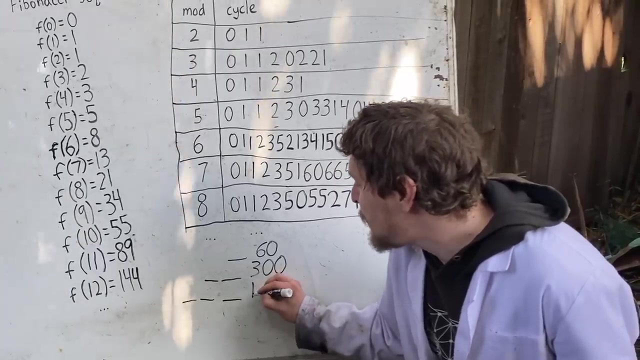 some fictional base 100 that had digit symbols for everything from 0 to 99. but since 100 is 10 squared, it can also tell us about two places worth in base 10.. similarly, if we looked at the cycle in mod is 10 cubed, that would be a cycle 1500 numbers in length and then it would Loop Back Around through. 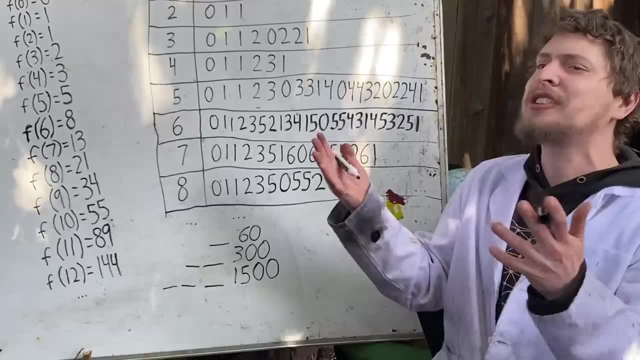 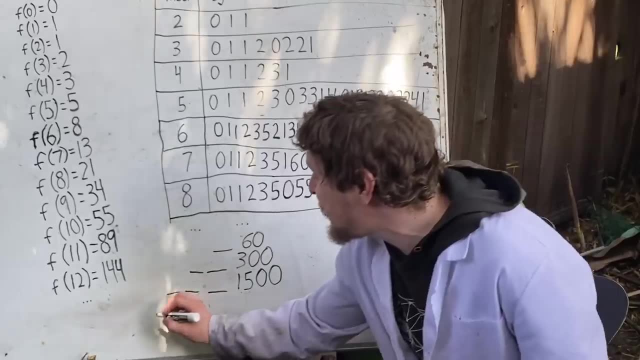 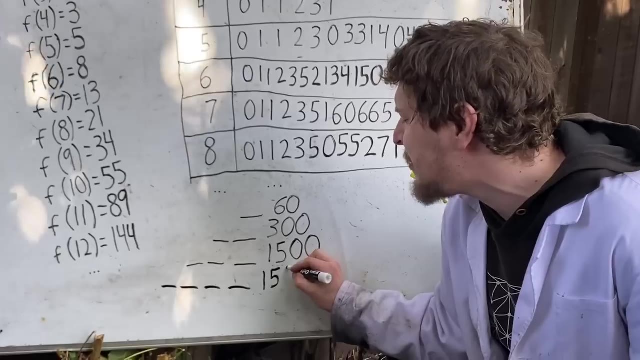 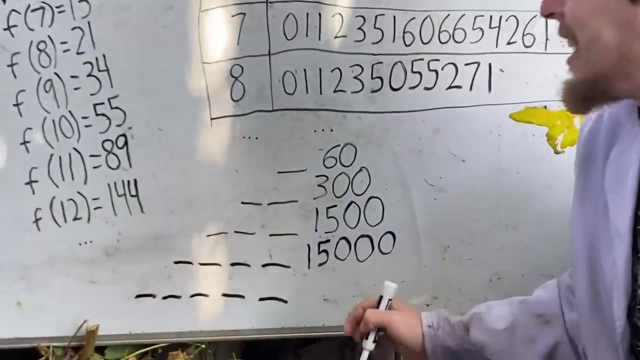 those numbers which could tell us about the last digit in some base 1 000 or the last three digits in base 10.. and we can continue, looking at mod 10 thousands pattern, which is fifteen thousand, looking kind of similar, And in fact to find mod 100,000, which would give us five digits worth in base 10,, that's 150,000.